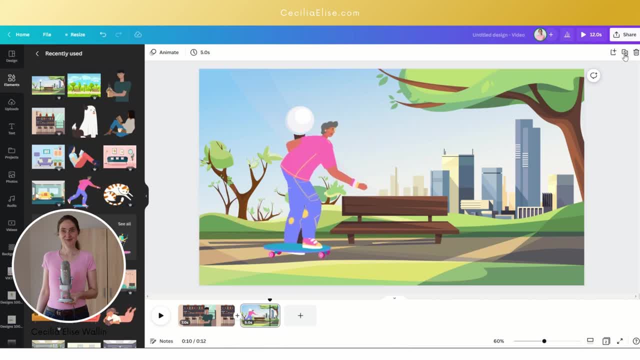 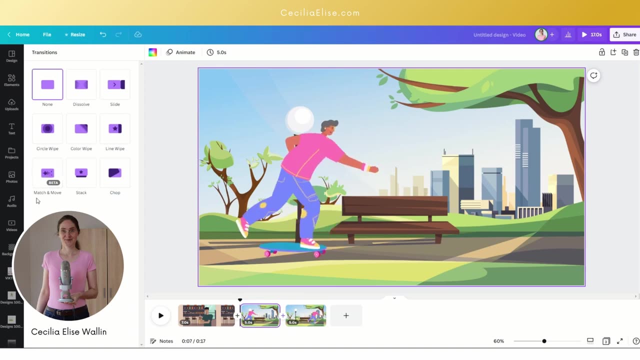 And we want the skater to move. so let's duplicate this frame and we are going to move the skater till here And now. we want to add a transition, a match and move transition, like this, so that the skater moves, and we want to make this frame much shorter, like this: 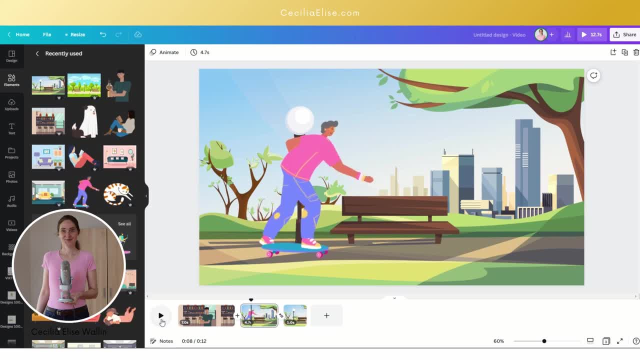 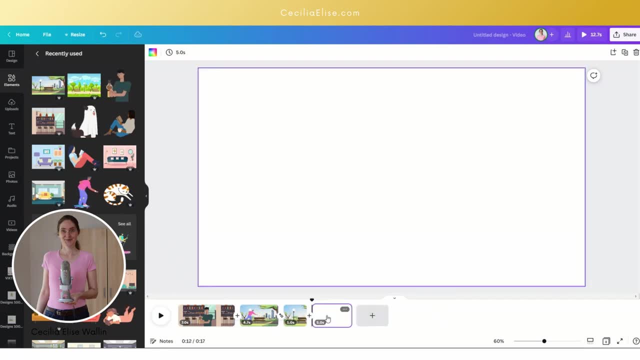 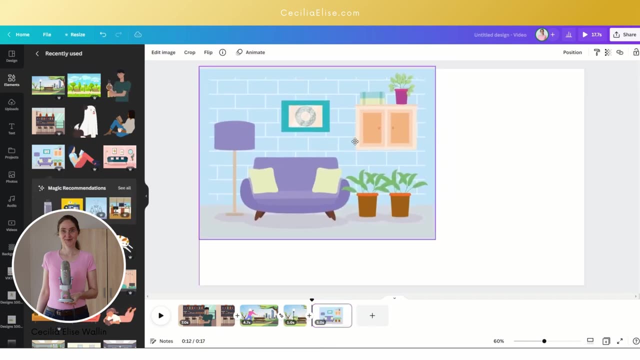 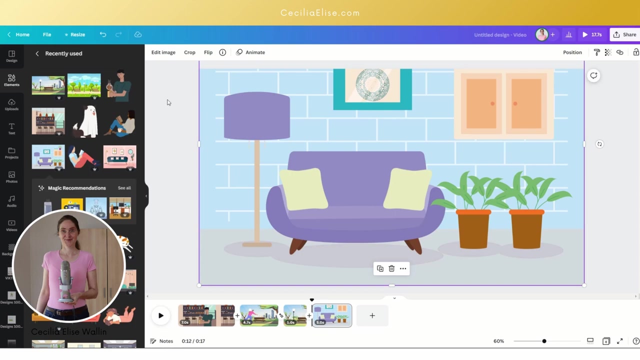 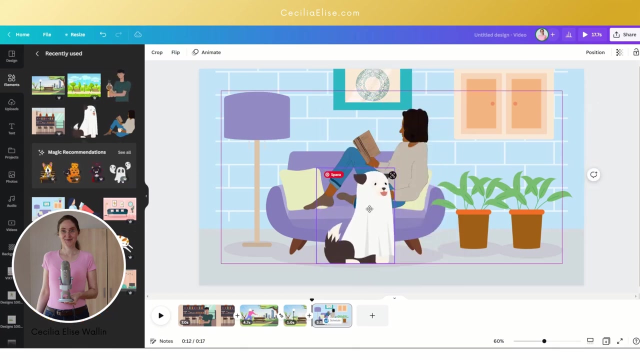 So let's see what this will look like here And now we want to add another frame, and here we want to have a living room like this, And we want to have someone sitting here in the sofa reading Like this, And we want to have an animation in this image as well, so we can search for an animated dog. 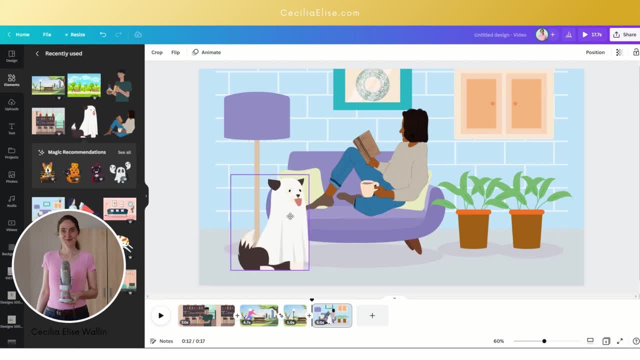 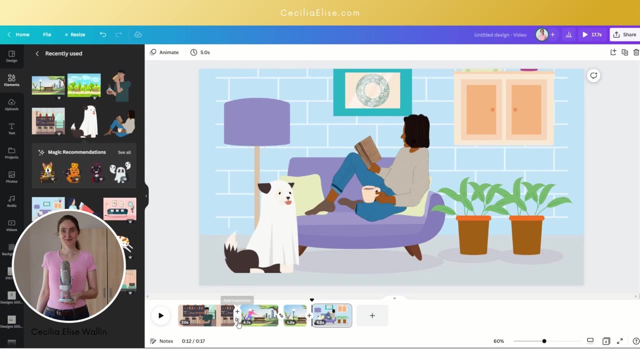 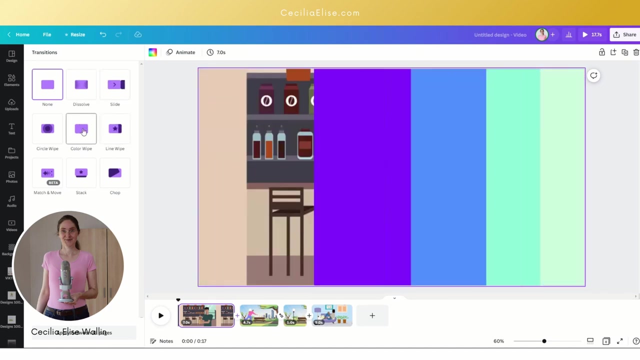 or cat, for example, like this: This is how you can create animated videos quickly in Canva. Now, before we export this brief video, we want to add beautiful transitions, so click here on add transition And you can choose from many different transitions here. Most of them look great. 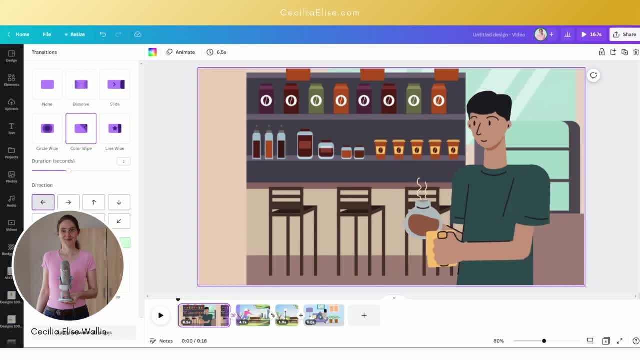 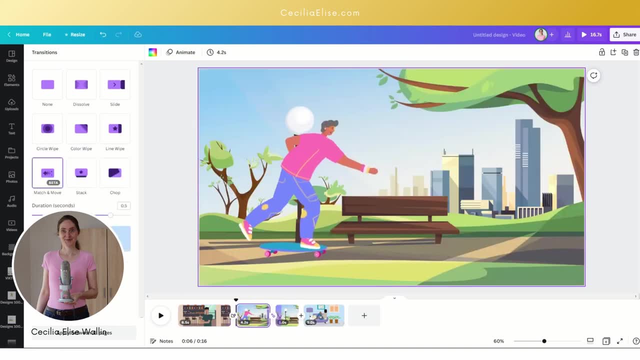 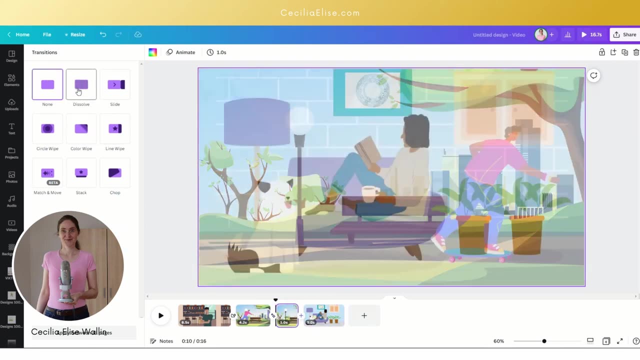 And here we can use the color wipe transition, And between these two frames we already have the match and move transition, because we want the skater to move like this And the last transition can be not dissolve, Maybe slide Or maybe line wipe. 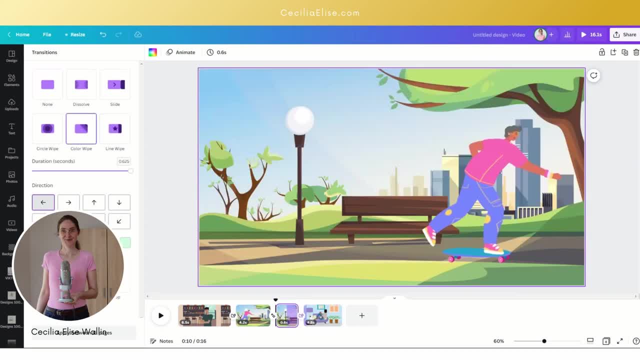 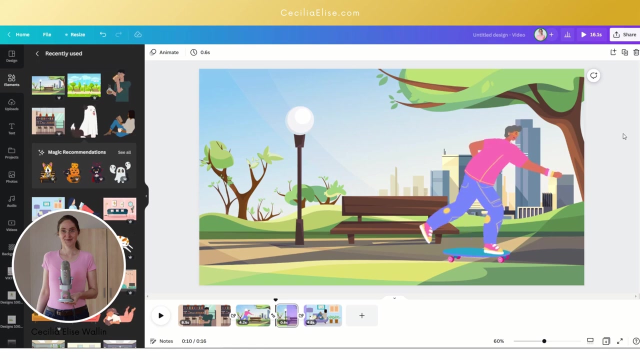 Or maybe a color wipe. again, We can change the colors of the color wipe here to any colors, so we can maybe change to some colors like this: Yeah, this looks good, And now we can export this brief video and now you can start creating really beautiful.